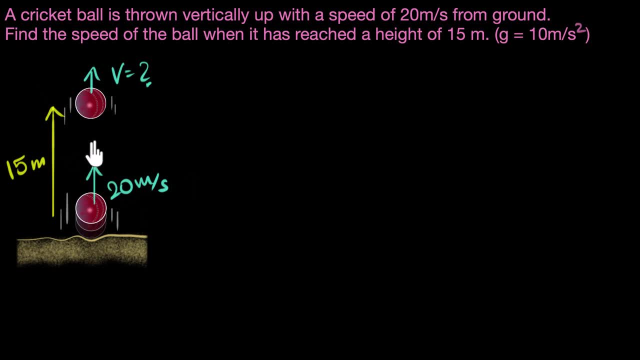 Now, as the ball goes up, its kinetic energy reduces, because the ball slows down, isn't it? But that kinetic energy gets converted to potential energy, because as the ball goes higher and higher, it has more and more potential energy. So, as a result, what we see is that 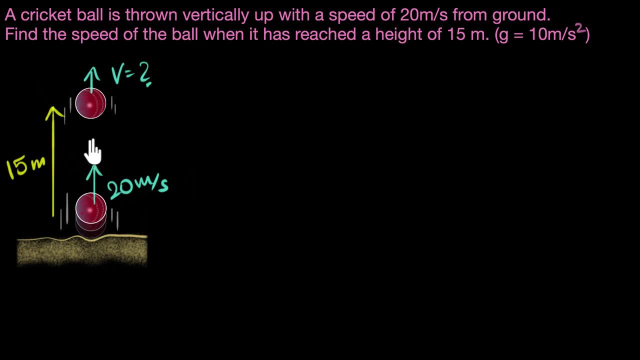 although the kinetic energy is reducing, potential energy is increasing and therefore the total energy does not change. That's the energy conservation principle. So we can now say that the total energy here should equal the total energy over here. okay, So mathematically we can say the total energy. 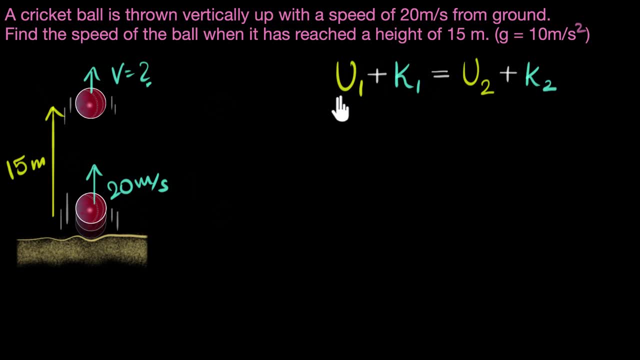 which is potential plus kinetic. u is for potential, okay, So potential plus kinetic at this point, which we can call, as you know, 0.1, that should equal the total energy over here. We can call this as 0.2.. 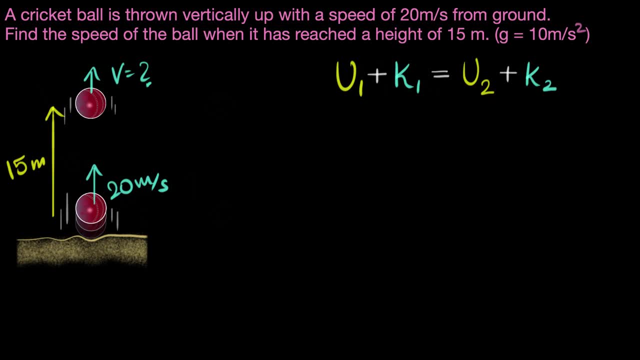 And then we can see if we can use this to try and solve our problem. So let's see, let's call this as point number one and let's call this as point number two. So we need to calculate the velocity at point number two, right? 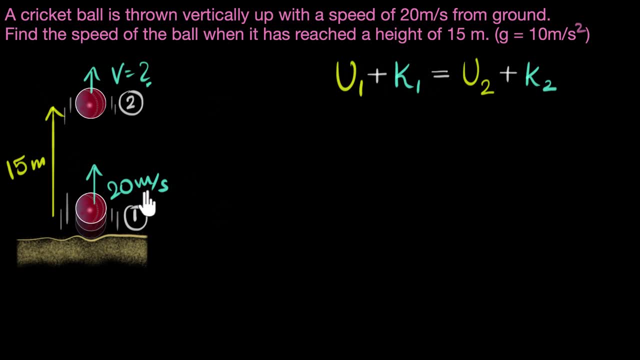 And here's the beautiful thing about this equation: I don't care which is initial and which is final. I could have called this as one and this as two. it doesn't matter. I can also use this equation if the ball is falling down. 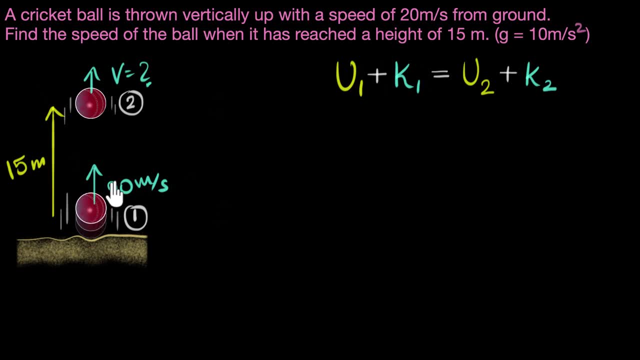 Even the direction doesn't matter over here. That's the beauty. I don't have to worry which is initial, which is final. Okay, so let's go ahead and substitute. Potential energy is mgh, because it's the potential energy to gravity, right. 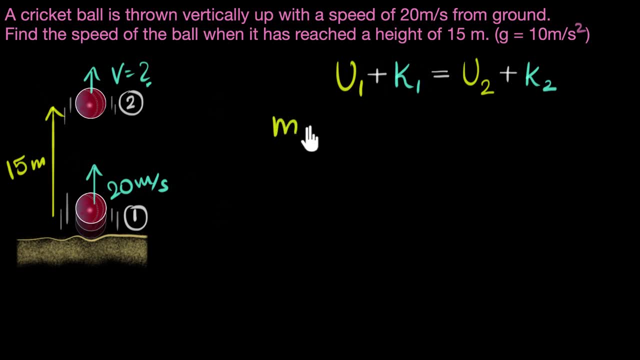 So over here, potential energy at one. we can say it is mgh one, where h one represents the height at this point Now. we'll substitute the values later, but let's just write it down now. So this will be mgh one. 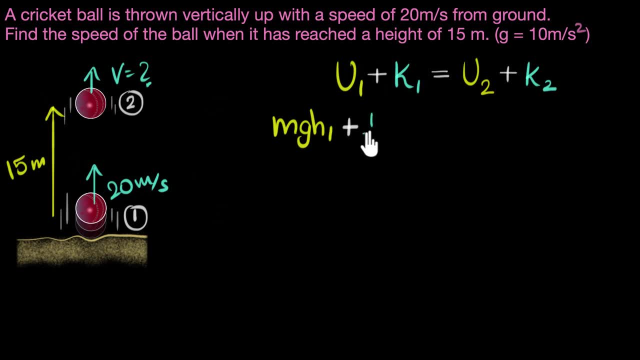 plus kinetic energy at point one would be half mv one squared, where v one would be the velocity at point one. So that should equal mgh two plus half mgh one mv two squared. Okay, now, before we substitute, can you see that m is common everywhere? 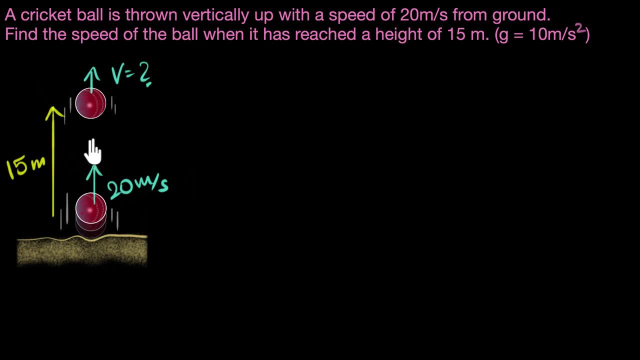 although the kinetic energy is reducing, potential energy is increasing and therefore the total energy does not change. That's the energy conservation principle. So we can now say that the total energy here should equal the total energy over here. okay, So mathematically we can say the total energy. 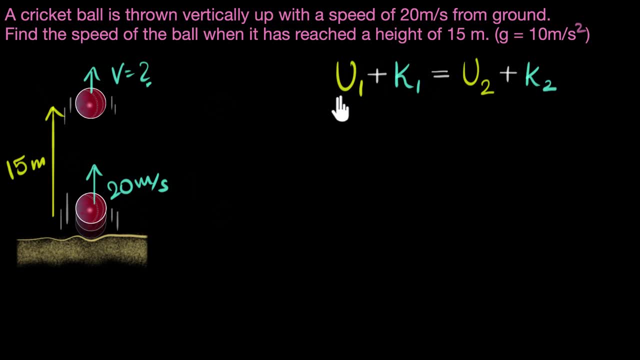 which is potential plus kinetic. U is for potential, okay, So potential plus kinetic at this point, which we can call, as you know, 0.1, that should equal the total energy over here. We can call this as 0.2.. 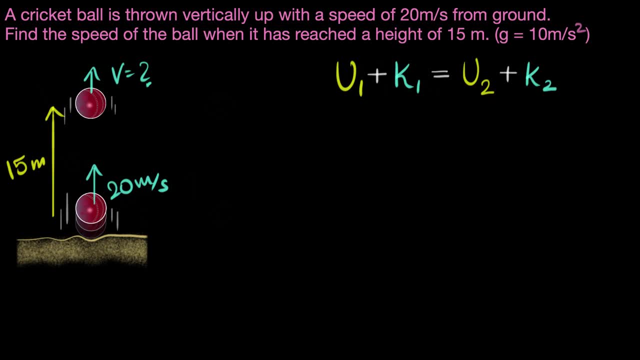 And then we can see if we can use this to try and solve our problem. So let's see, let's call this as point number one and let's call this as point number two. So we need to calculate the velocity at point number two, right? 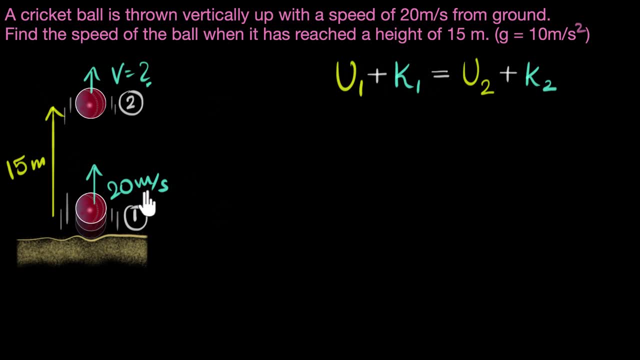 And here's the beautiful thing about this equation: I don't care which is initial and which is final. I could have called this as one and this as two. it doesn't matter. I can also use this equation if the ball is falling down. 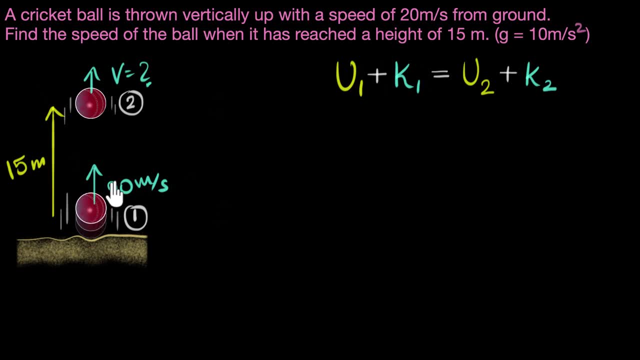 Even the direction doesn't matter over here. That's the beauty. I don't have to worry which is initial, which is final. Okay, so let's go ahead and substitute. Potential energy is mgh, because it's the potential energy to gravity, right. 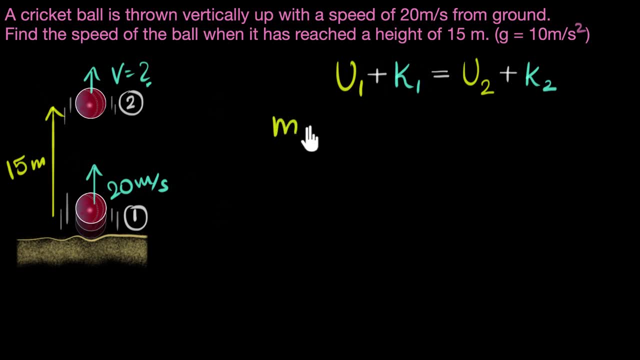 So over here, potential energy at one. we can say it is mgh one, where h one represents the height at this point Now. we'll substitute the values later, but let's just write it down now. So this will be mgh one. 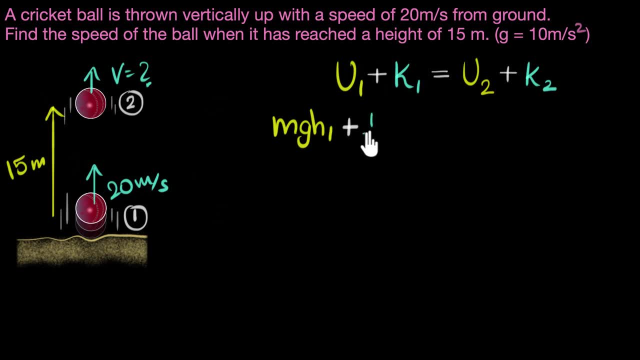 plus kinetic energy at point one would be half mv one squared, where v one would be the velocity at point one. So that should equal mgh two plus half mgh one mv two squared. Okay, now, before we substitute, can you see that m is common everywhere? 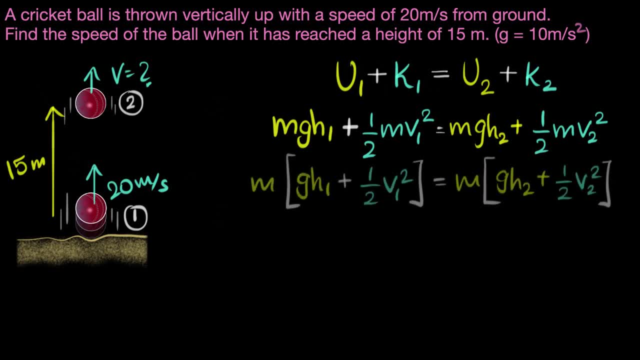 Let's pull that out. So if we take m common, then you see m cancels out. And now let's see if we have everything that we want. We know the value of g, that's given H one. what is h one? 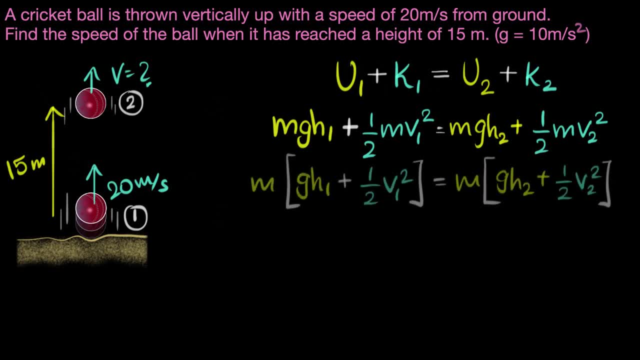 Let's pull that out. So if we take m common, then you see m cancels out. And now let's see if we have everything that we want. We know the value of g, that's given H one. what is h one? 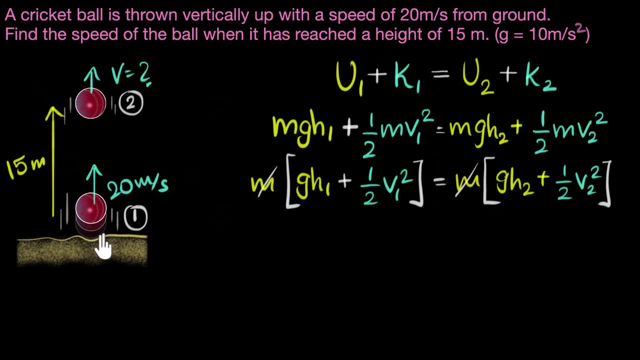 H one is the height. at this point We know that It's zero, right, Because I'm throwing from the ground. So I know h one is zero. I know v one, that is, this number. H two, oh, I know h two. 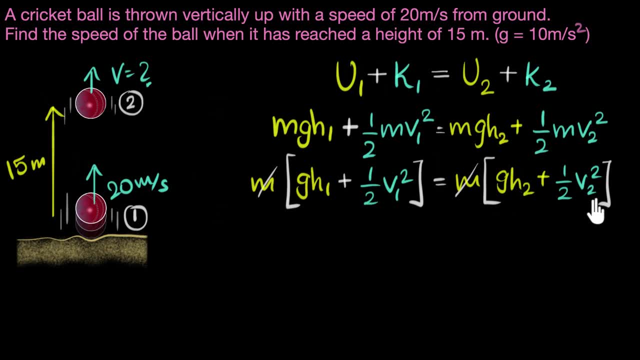 that is the height at this point. that is 15 meters, Which means I need to calculate what v two is, And that's the only thing I can. that's the only unknown over here, So I can just plug in and calculate. 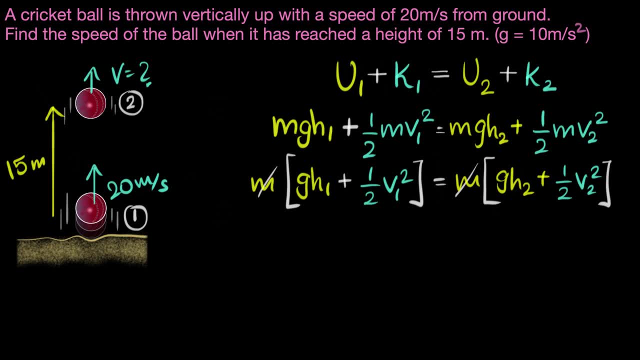 So you know what Great idea to pause the video and see if you can substitute and get the answer yourself. Okay, let's substitute. So h one is zero. Therefore, this will be zero plus half half v one squared, What is v one? 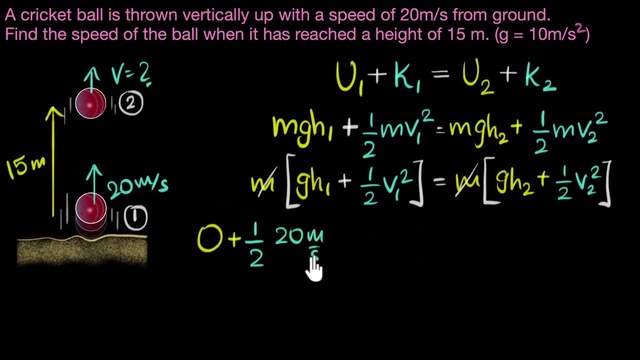 v one is velocity at this point, So it's 20 meters per second squared. That should equal g times h two. G is given 10 meters per second squared times h two. H two is 15 meters Plus half v two squared. 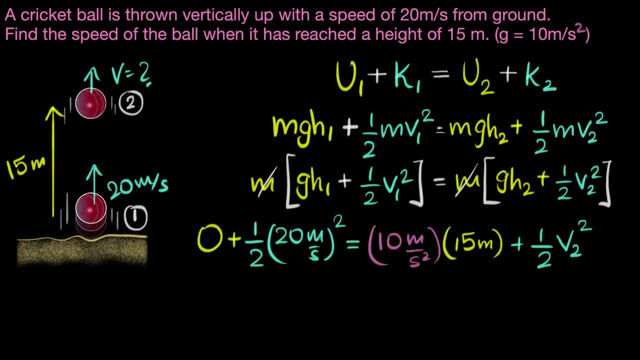 I don't know. v two: I need to figure that out. Okay, so let's see what we get: 20 squared is 400.. 400 divided by two is 200. So let me write that directly. So I get 200 on the left-hand side. 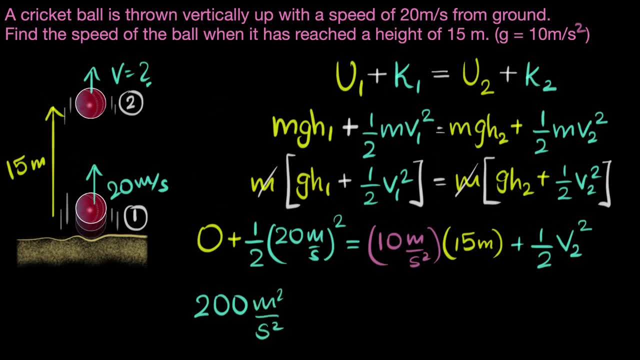 meters squared per second squared, And that equals- let's see what I get here: 10 into 15 is 150.. Okay, So I get 150.. Again, meters squared per second squared. Oops, second squared Plus half v two squared. 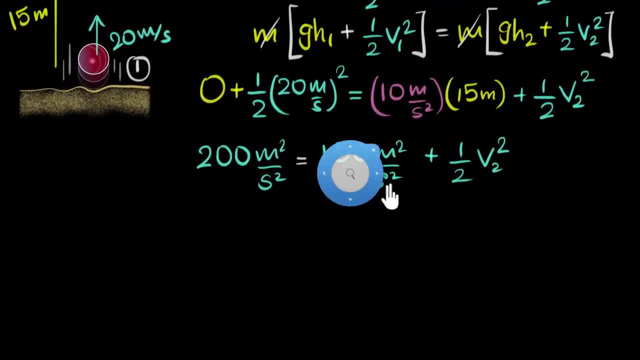 Okay, let's move down so that we can make some space. Now, since I want what v two is, let's subtract 150 on both sides, So now I'll get 200 minus 150 on the left-hand side, And that gives me 50.. 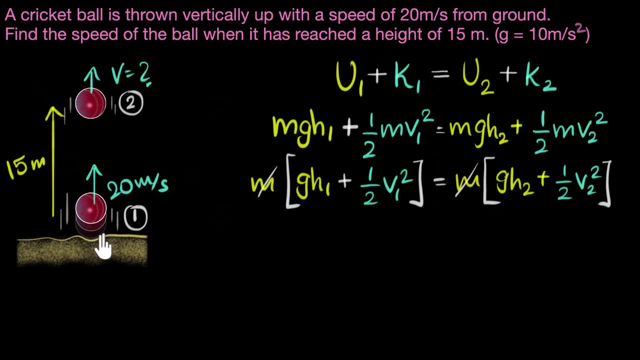 H one is the height. at this point We know that It's zero, right, Because I'm throwing from the ground. So I know h one is zero. I know v one, that is, this number. H two, oh, I know h two. 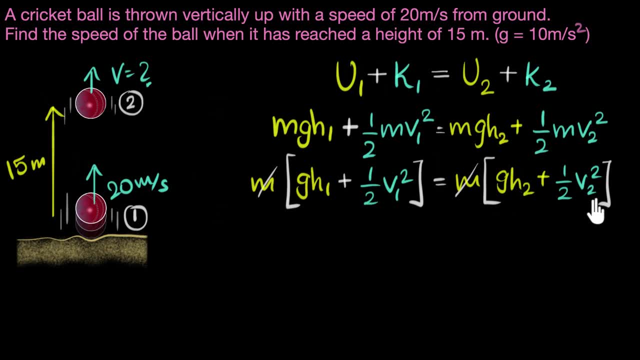 that is the height at this point. that is 15 meters, Which means I need to calculate what v two is, And that's the only thing I can. that's the only unknown over here, So I can just plug in and calculate. 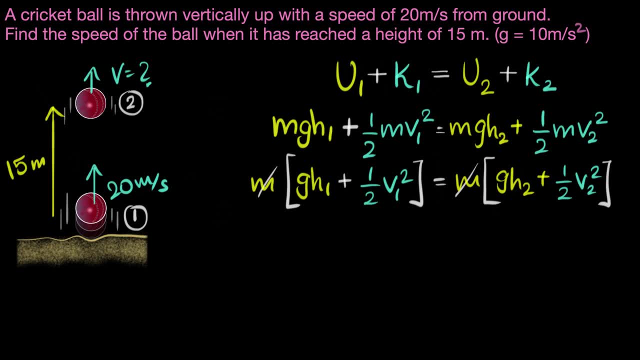 So you know what Great idea to pause the video and see if you can substitute and get the answer yourself. Okay, let's substitute. So h one is zero. Therefore, this will be zero plus half half v one squared, What is v one? 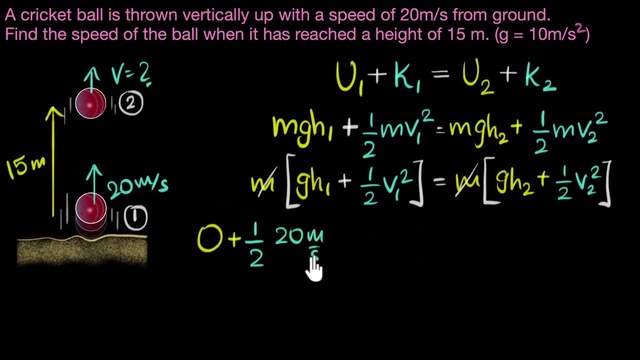 v one is velocity at this point, So it's 20 meters per second squared. That should equal g times h two. G is given 10 meters per second squared times h two. H two is 15 meters Plus half v two squared. 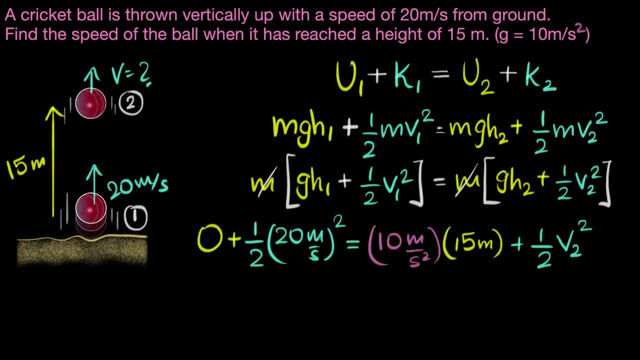 I don't know. v two: I need to figure that out. Okay, so let's see what we get: 20 squared is 400.. 400 divided by two is 200. So let me write that directly. So I get 200 on the left-hand side. 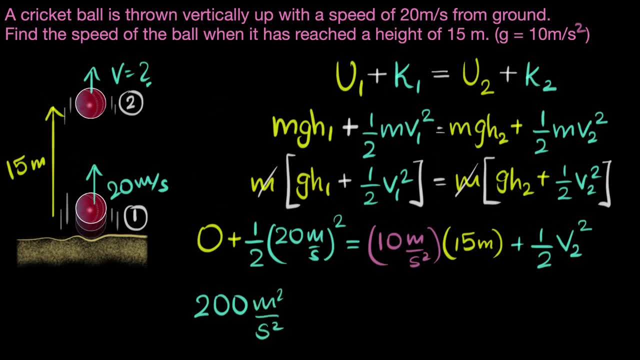 meters squared per second squared, And that equals- let's see what I get here: 10 into 15 is 150.. Okay, So I get 150.. Again, meters squared per second squared. Oops, second squared Plus half v two squared. 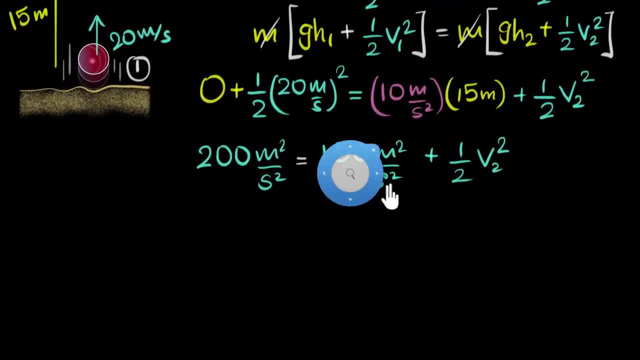 Okay, let's move down so that we can make some space. Now, since I want what v two is, let's subtract 150 on both sides, So now I'll get 200 minus 150 on the left-hand side, And that gives me 50.. 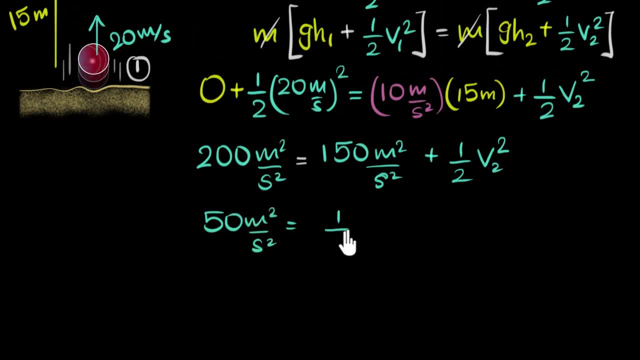 50 meters squared per second squared On the left side. That equals half v two squared And if I multiply by two on both sides I will get 100 meters squared per second squared equals v two squared. And since I want what v two is, 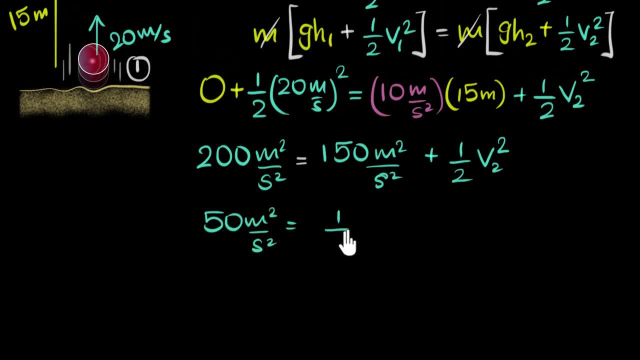 50 meters squared per second squared On the left side. that equals half v two squared And if I multiply by two on both sides I will get 100 meters squared per second squared equals v two squared. And since I want what v two is, 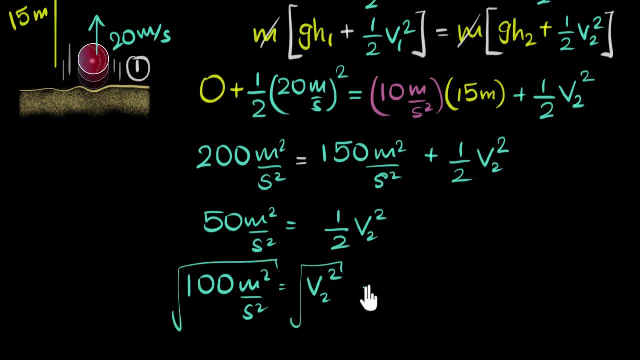 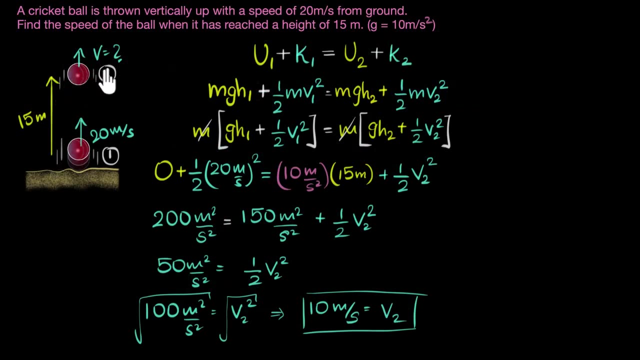 I can just take the square root on both sides And that gives me square root of 100 is 10.. 10 meters per second equals v two. There's our answer. And so when the ball reaches the height of 15 meters, its velocity would be 10 meters. 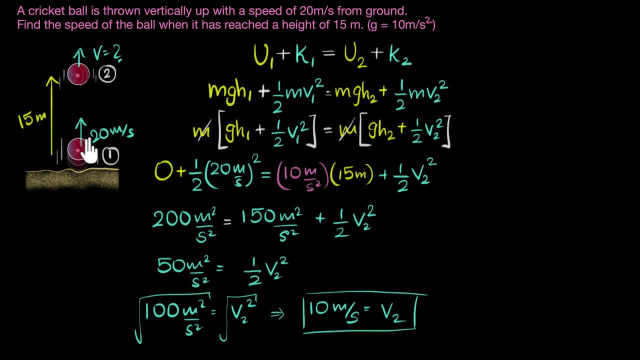 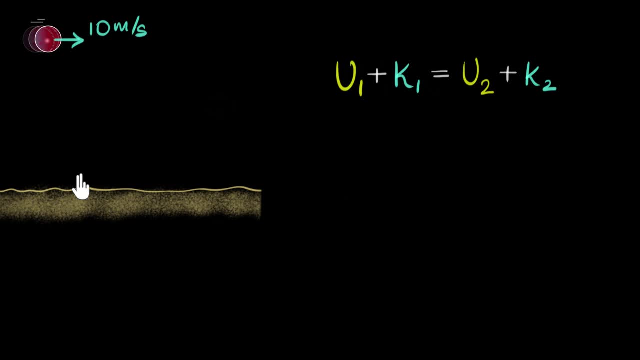 per second. It's slower, it has become slower and that's what we would predict. Alright, let's solve one more In this problem. we'll directly look at the diagram. okay, So we have a ball that's being thrown horizontally at 10 meters per second from a height of 40. 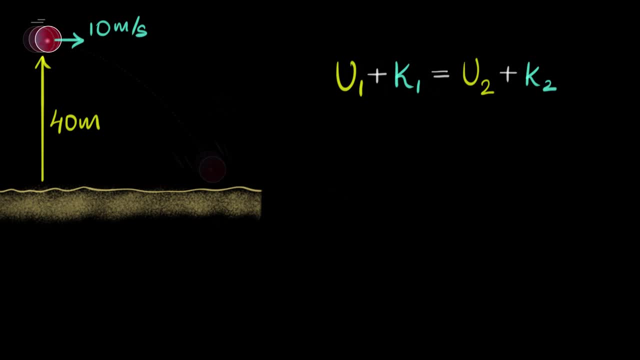 meters from the ground. okay, So the ball is going to go in some kind of a curved path, And the question now is: with what speed will that ball go and hit the ground? Okay, so how do we calculate this velocity? At first this problem does look a little complicated, because you see here the ball. 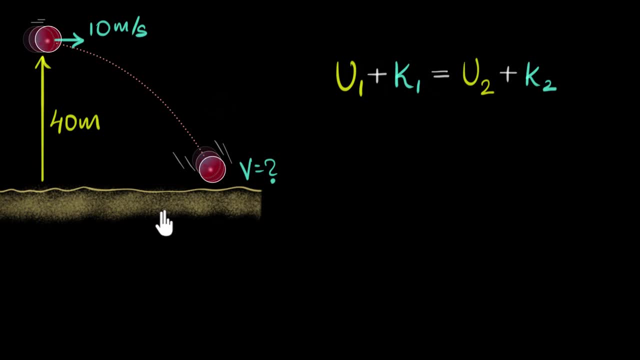 is going in a curved path, So there is direction changing and everything right, But energy conservation doesn't care about directions. okay, So even if the ball is going in a curved path, This principle works. So all we have to do is say: total energy here should equal total energy over here, and we 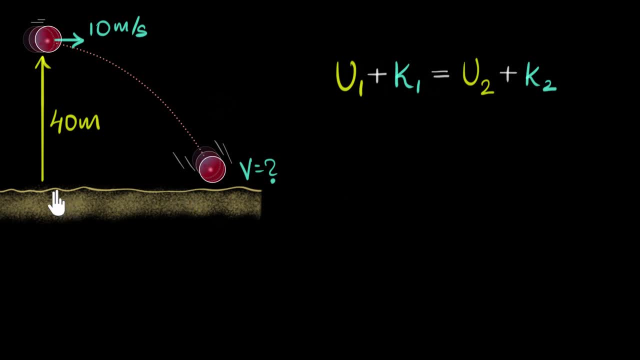 can solve it. So great idea to pause the video and see if you can try and solve this yourself first. Okay, so again, let's call this as position one, Let's call this as position two And, just like before, let's write down the values. 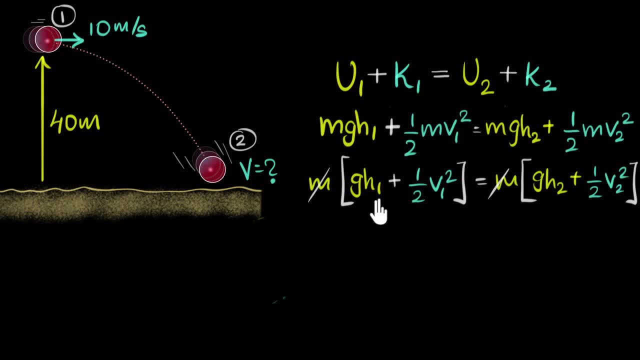 So the initial steps will all be the same. Let's just look at what our H and V values will be. H1 would be the height at point one, that is 40. So we know that V1 is also something we know, that's 10.. 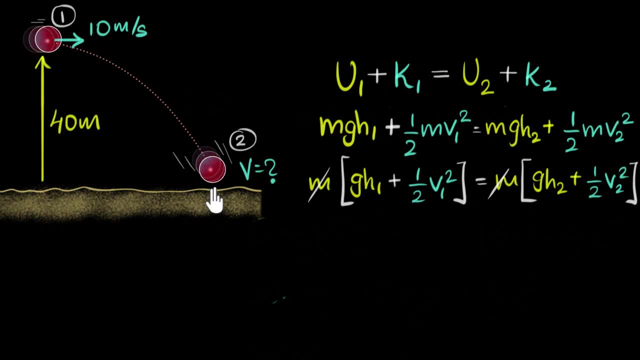 H2 is the height at point two, which is zero in this case. V2 is the velocity at point two. That's what we want to calculate. So V2 is again what we want to figure out. So let's go ahead and substitute. 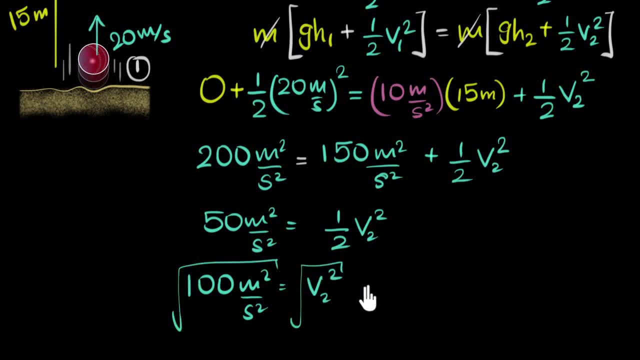 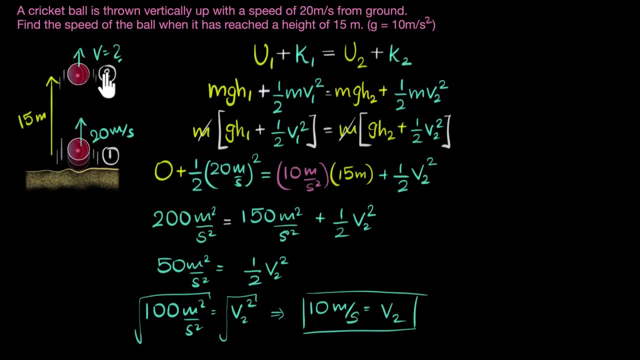 I can just take the square root on both sides And that gives me square root of 100 is 10.. 10 meters per second equals v two. There's our answer. Okay, And so when the ball reaches the height of 15 meters, its velocity would be 10 meters. 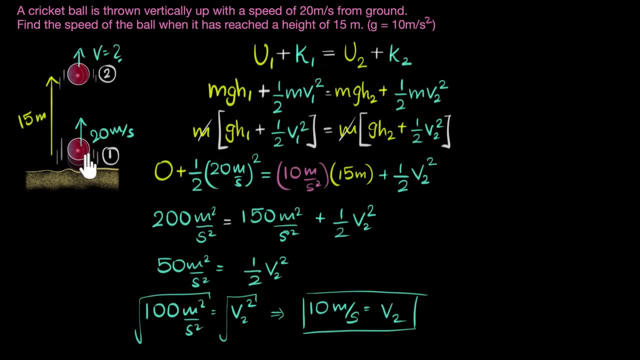 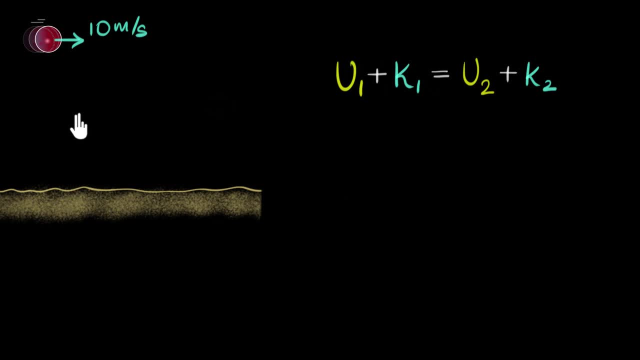 per second. It's slower, it has become slower and that's what we would predict. Alright, let's solve one more In this problem. we'll directly look at the diagram. okay, So we have a ball that's being thrown horizontally at 10 meters per second from a height of 40. 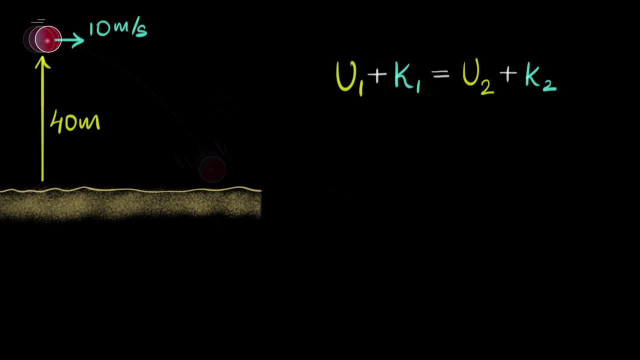 meters from the ground. okay, So the ball is going to go in some kind of a curved path, And the question now is: with what speed will that ball go and hit the ground? Okay, so how do we calculate this velocity? At first this problem does look a little complicated, because you see here the ball. 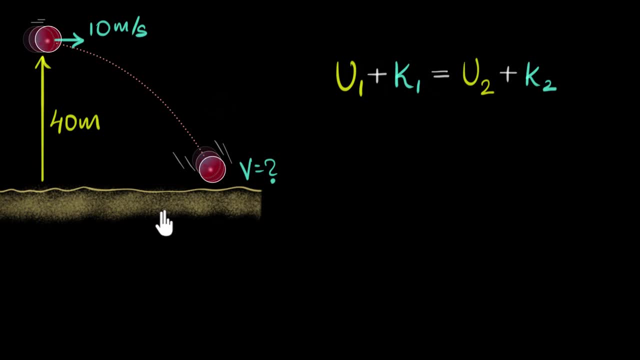 is going in a curved path, So there is direction changing and everything right, But energy conservation doesn't care about directions. okay, So even if the ball is going in a curved path, This principle works. So all we have to do is say: total energy here should equal total energy over here, and we 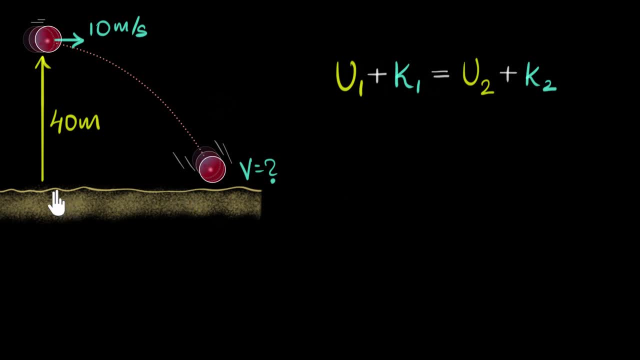 can solve it. So great idea to pause the video and see if you can try and solve this yourself first. Okay, so again, let's call this as position one, Let's call this as position two And, just like before, let's write down the values. 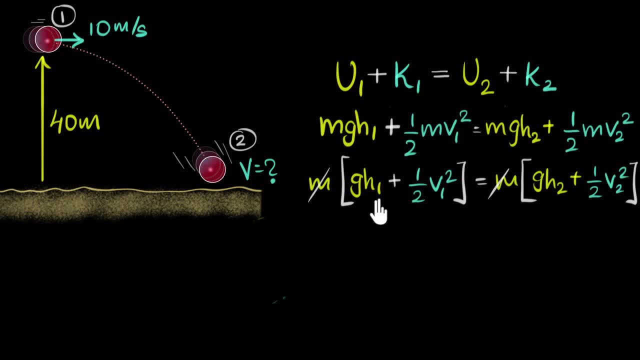 So the initial steps will all be the same. Let's just look at what our H and V values will be. H1 would be the height at point one, that is 40. So we know that V1 is also something we know, that's 10.. 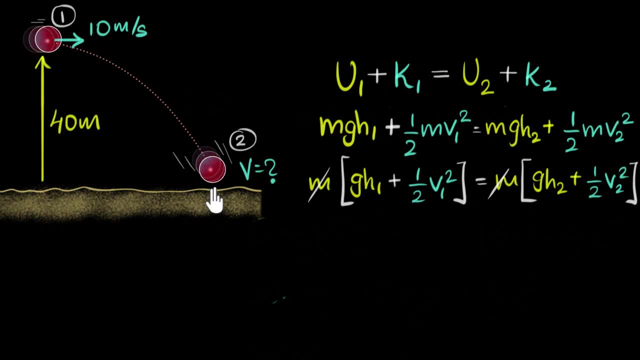 H2 is the height at point two, which is zero in this case. V2 is the velocity at point two. That's what we want to calculate. So V2 is again what we want to figure out. So let's go ahead and substitute. 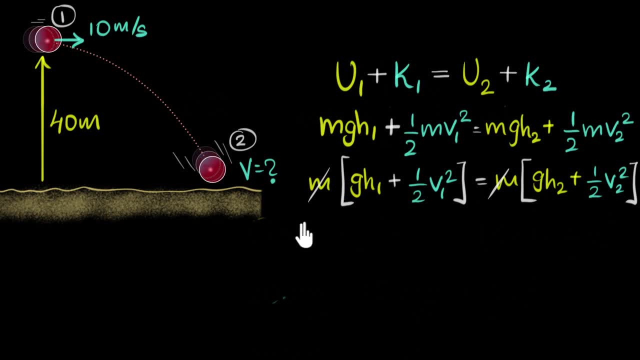 Again, let's take G as 10 itself, So it'll be 10 meters per second square times H1.. This time is 40 meters Plus half V1 squared. V1 is 10 meters per second the whole squared.